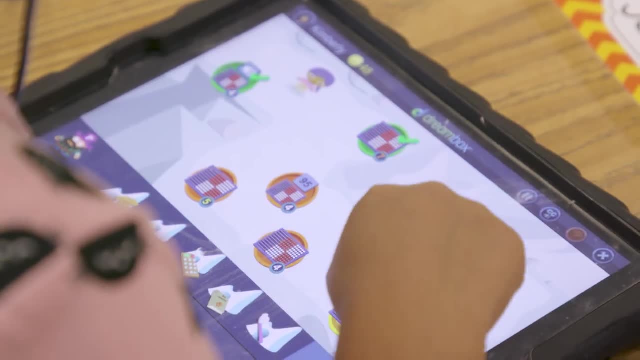 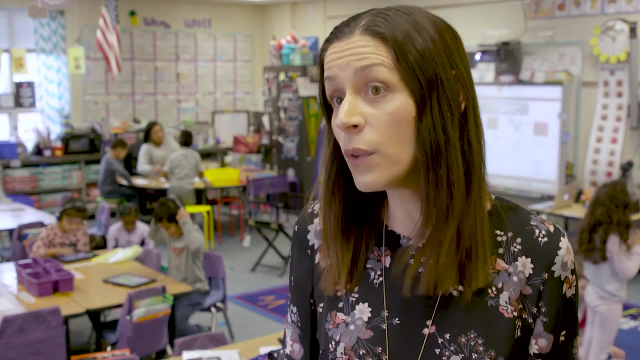 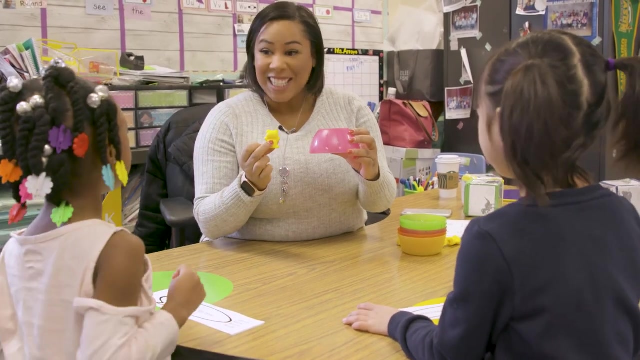 promote growth. So a common theme that you see in all schools that use Math Workshop is student autonomy. It was students making selections about what they're doing and thinking about their goals and what they need to work on in order to improve. Where's the bear Next, Next to Next? to Go ahead and read it. 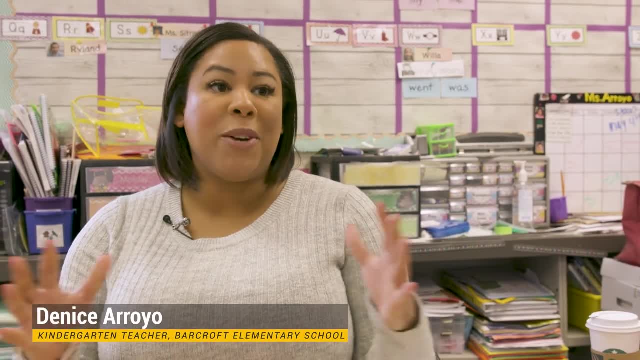 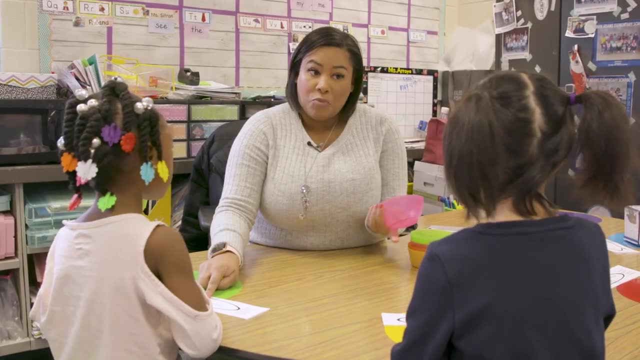 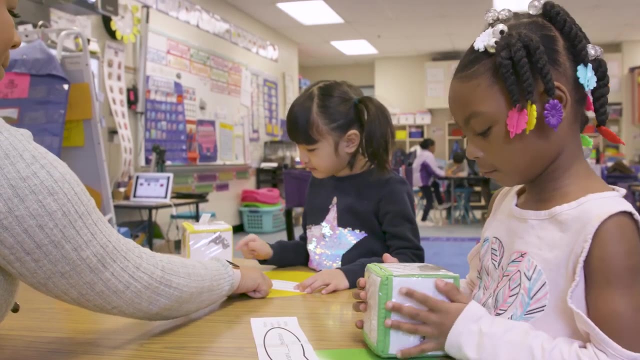 So we just had a kindergarten mid-year math assessment. Upon reviewing that data, I realized that the students needed more practice on position words. So today we did a whole group mini lesson on that. So I called them over today and I explained to them the position words that we're working. 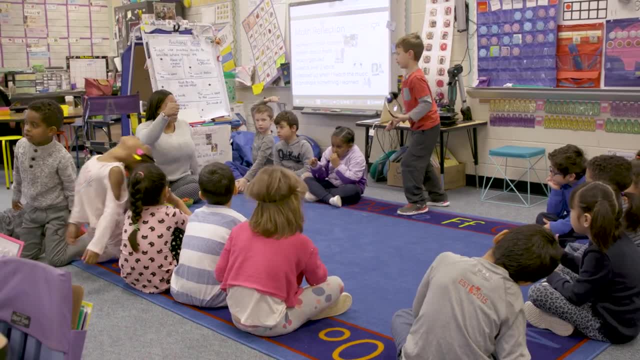 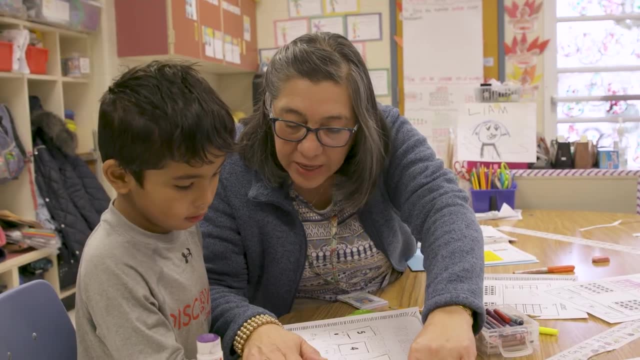 on It's super data-driven. I mean, if they prove to me that they understand it on paper and they understand it with me in a performance test, then I know that they have understanding of that standard. And if they can't show that, then I know through Math Workshop that I have. 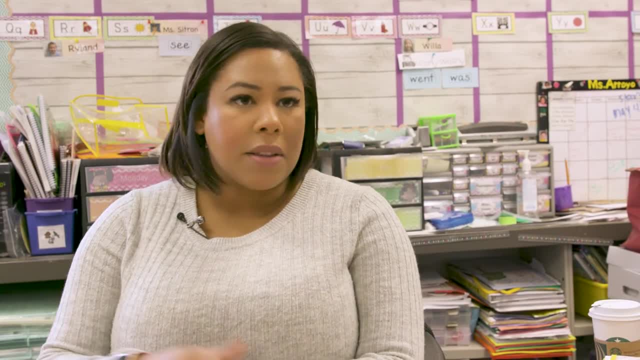 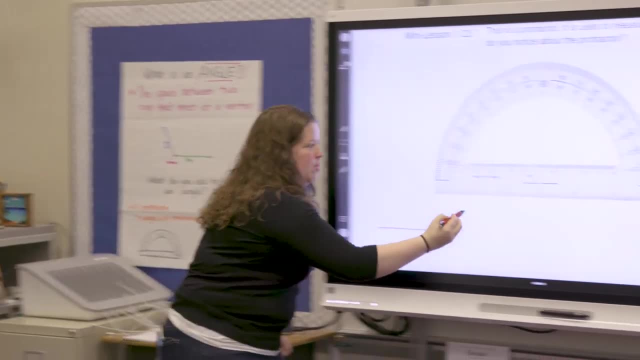 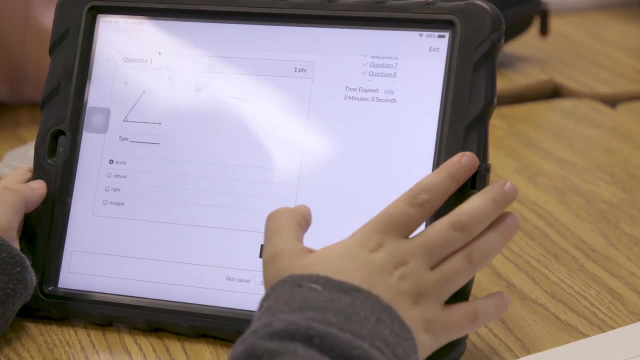 the flexibility to continue working with them however long they need to, And so if we have an angle and we line it up here, we need to measure the inside right. Our choice board in this classroom is on Canvas, and that allows me to incorporate video explanations. 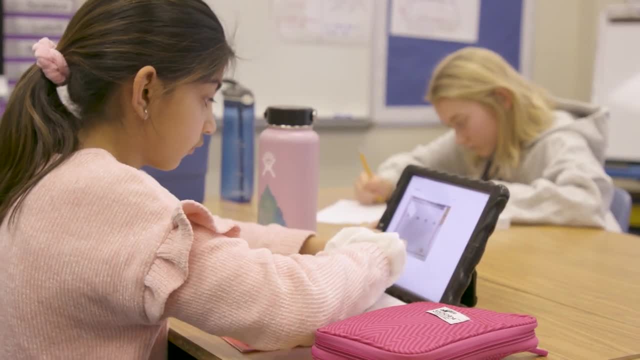 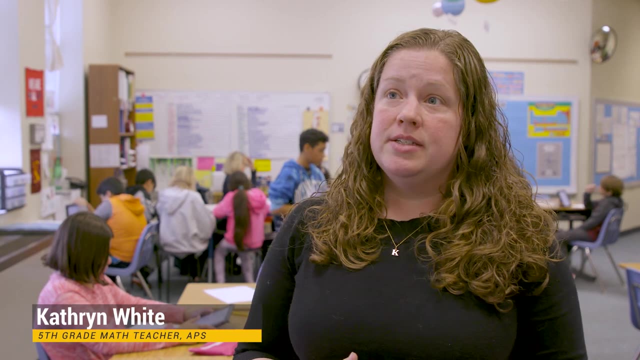 where I can demonstrate strategies or explanations of the activity. They can make videos themselves, sometimes, of things that they've done and then they can upload those for me to see, and that kind of is another way for them to demonstrate their understanding, If it's a worksheet. 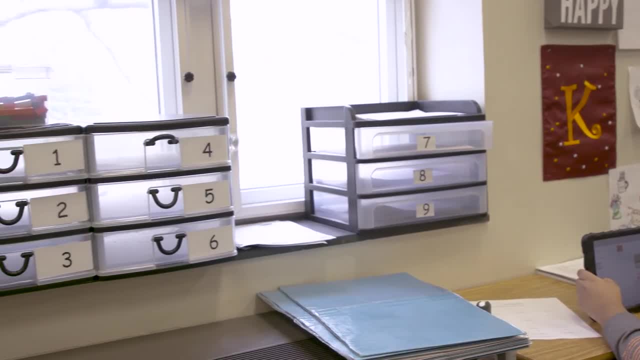 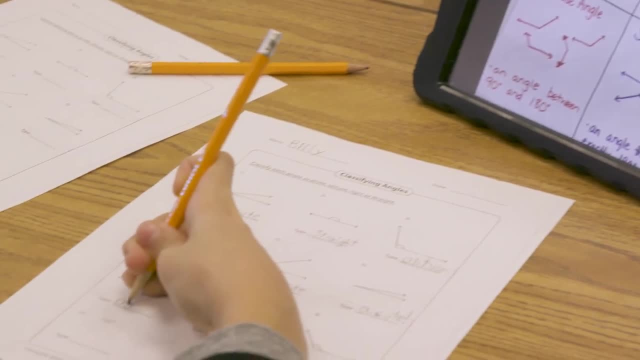 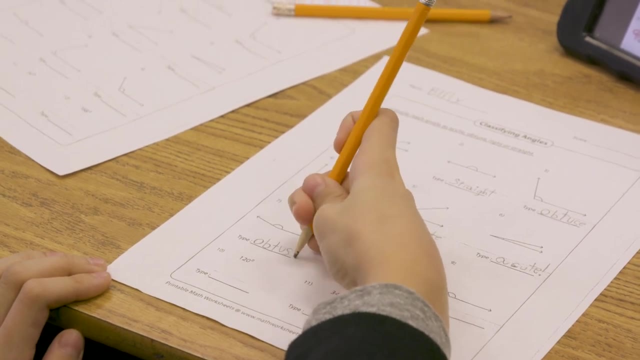 based activity. I have drawers in the classroom that are numbered so that students can go and find that and everything is scored in Canvas. So it kind of takes a layer of work off of me so that they get instant feedback of how they did or what they need to fix. 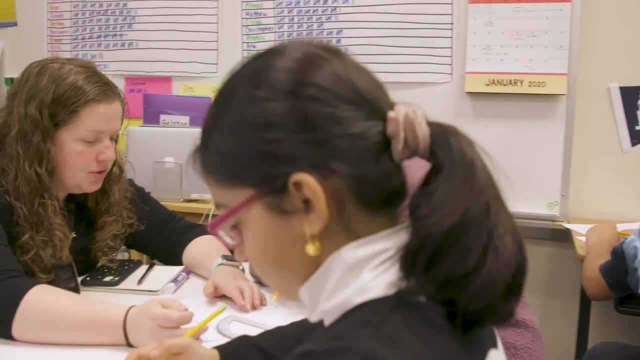 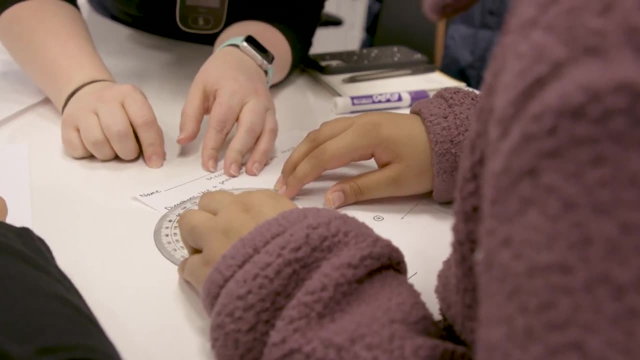 They have videos they can go watch if they need to practice that strategy again, and then they can try it again, And that way I don't have to grade the work. They've gotten instant feedback and they have tools that they're familiar with. I can use my fingertips to help them. 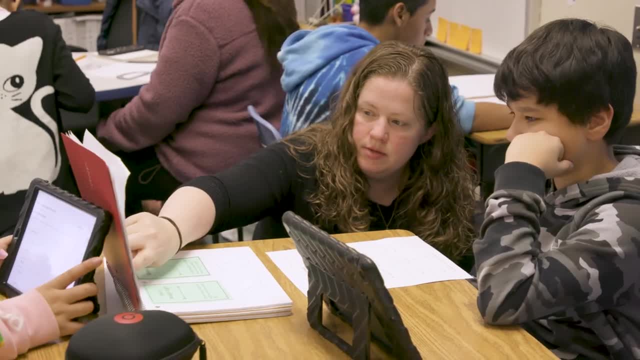 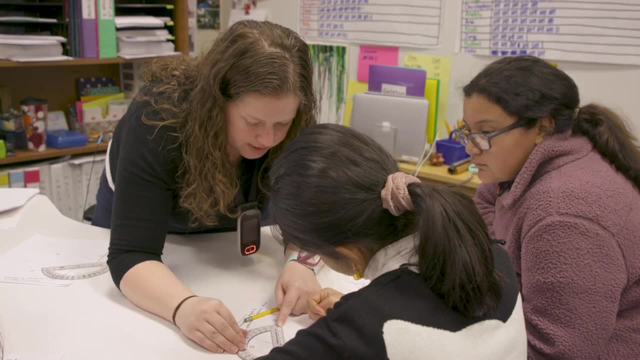 So the reflection at the end is usually a way for me to try to ensure that students have gotten out of the lesson what I was hoping for them to get out of it. It also allows me to see if they didn't, and maybe they got something else out of it, or maybe there's.